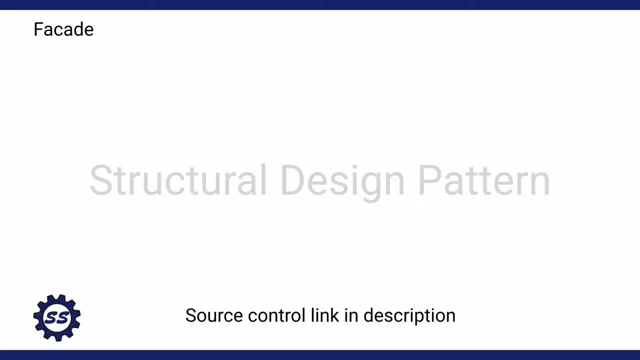 The facade design pattern is a structural design pattern that takes multiple subsystems of our package and unifies them in a simple, easy to use interface for the client. Now, this is especially important because the client shouldn't have to know about or understand how all the subsystems 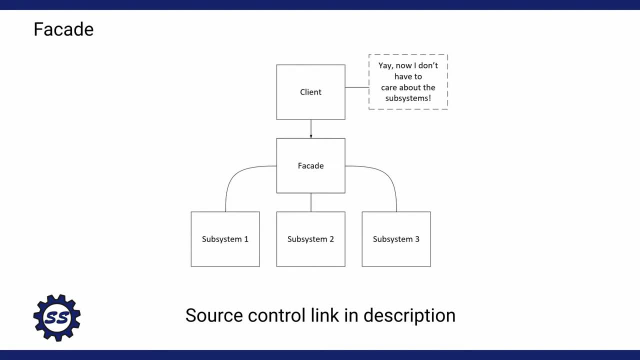 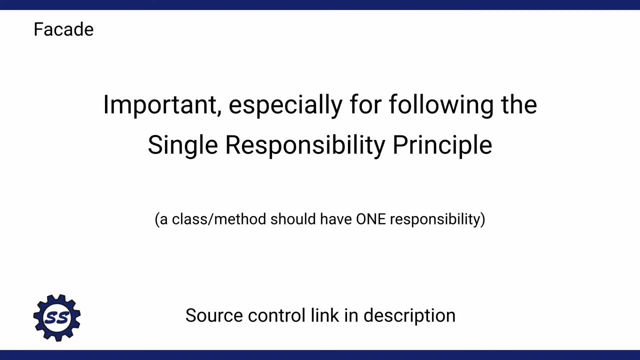 interact together. It should just get the unified interface that'll perform the functionality that it ultimately wants to perform and the client won't be doing too much. I believe this pattern is pretty important and we're going to see this in the demo. but, for example, you hear a lot in the 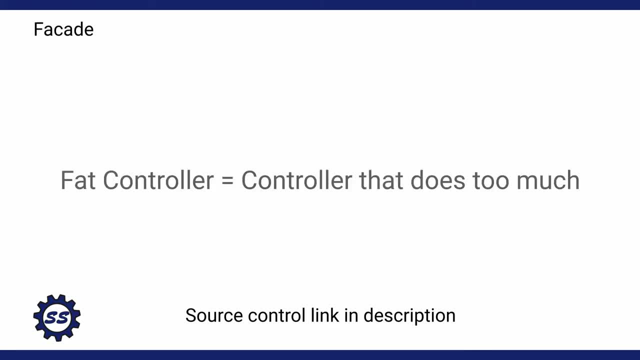 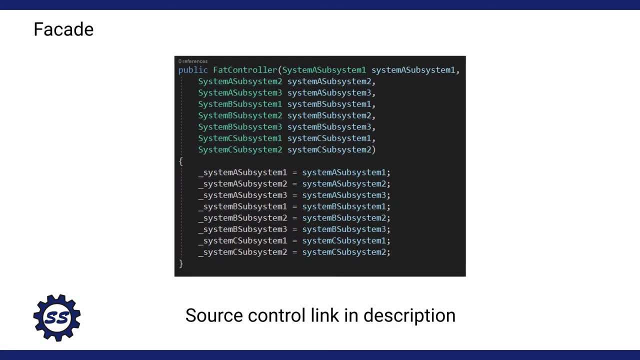 ASPNET community about trying to remove fat controllers or controllers that do too much have. massive constructors have just lots of lines in the file. They're taking too many subsystems and doing all the logic within the controller. Ideally, those subsystems should be moved into a 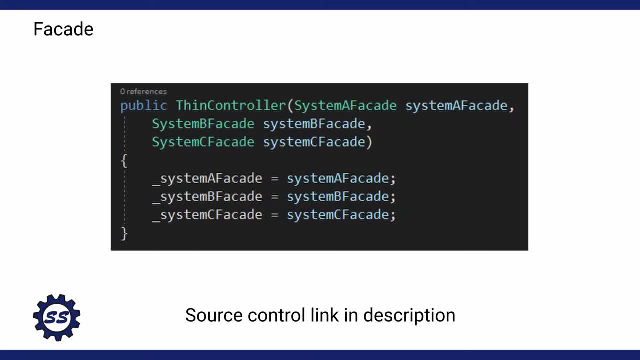 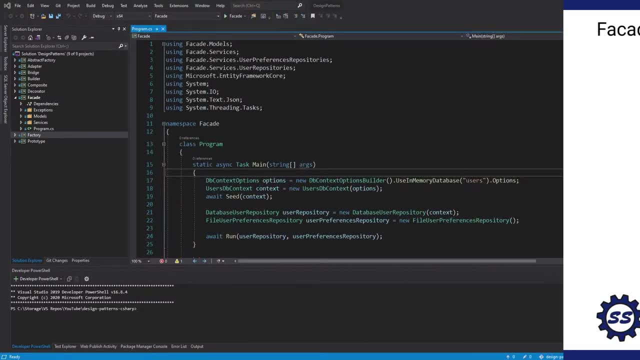 facade, and then the controller only has to know about the facade, which is going to do all the work. So that's just one place where I could see the facade pattern being useful, but there's many others and hopefully this demo will inspire you to do that. 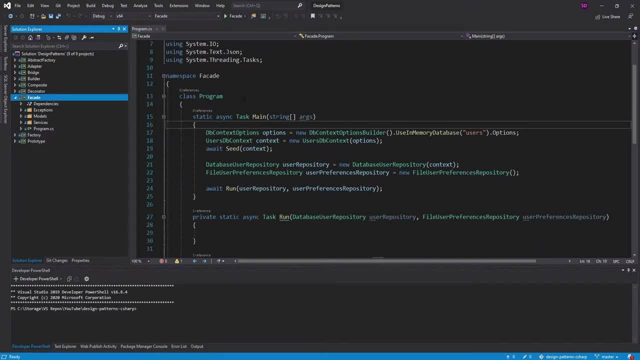 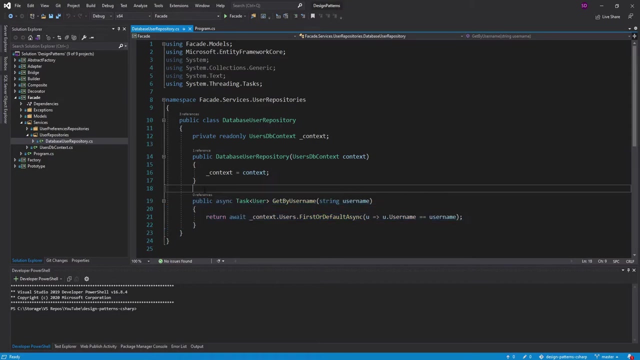 So here in this demo I have a couple of subsystems and the first subsystem I have is a user repository and we can see that in the services folder I have user repositories and this just interacts with my entity framework database and gets users for me. 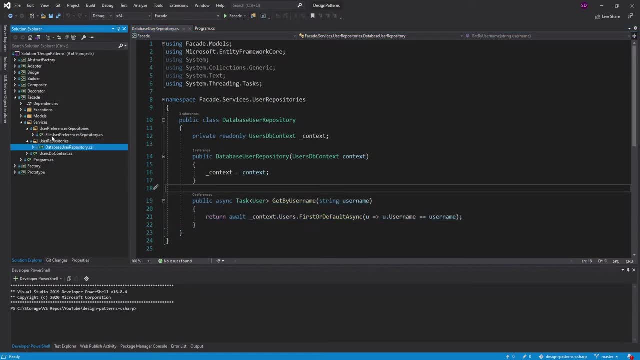 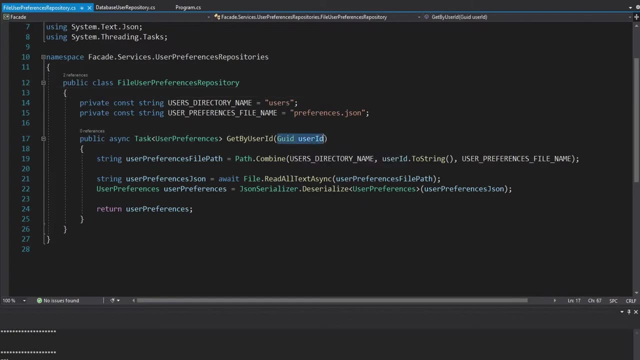 The other subsystem is my user preferences repository, and right now I have this implemented using a file and what we can do is we can get a user's preferences by the user id and this simply opens up a preferencesjson file that I have in my directory and if we look at user preferences, it, 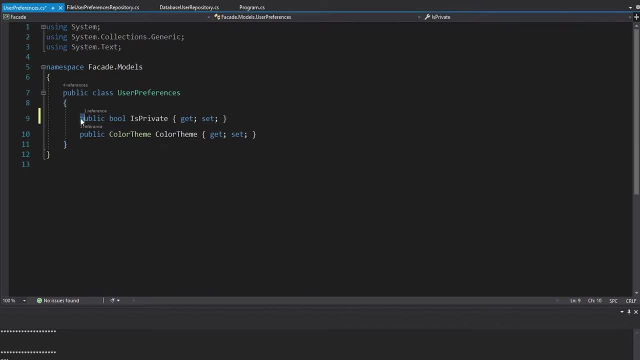 just has some things like if the user's profile is private and also their color scheme for their profile as well. so light, blue, dark. basically just rip those out of visual studio and we can also look at the user. so I didn't go over this. but a user just has an id which we'll use to get the 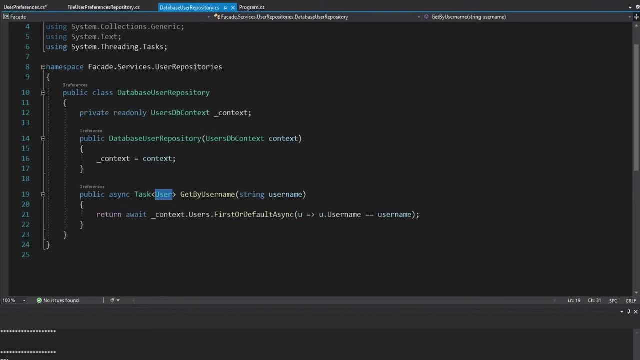 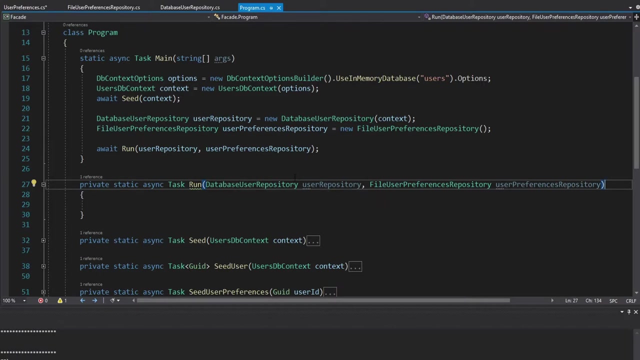 user preferences, an email and a username. So pretty basic application, but the main idea here is that we have two subsystems, One to get users and another subsystem to get the user preferences. Anyways, let's look at this run method. so this takes two parameters, one for each of my subsystems. 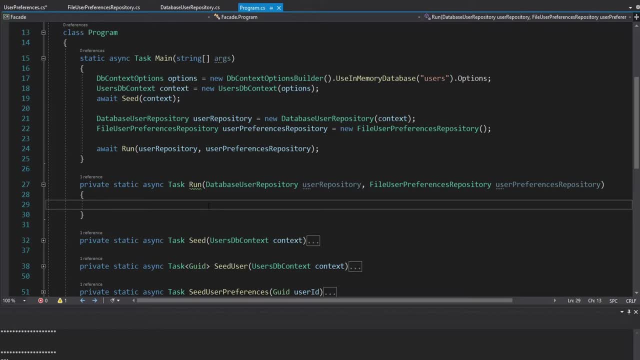 so we're going to implement our logic for the application in this run method and what I want to do is first get a user. so we'll use our user repository and get by username. but the user I want to get is singleton sean, and this is all a single weight. so we will await this and put it into a user. 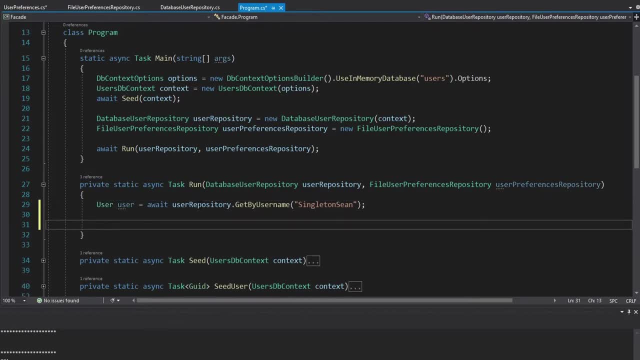 variable, Then I want to get the preferences for that user, so I will use my user preferences repository, get the preferences by user id. we can pass in our user id- very convenient, and we have to await this as well and put that into a user preferences. and now part of the logic of my application, I want to check. 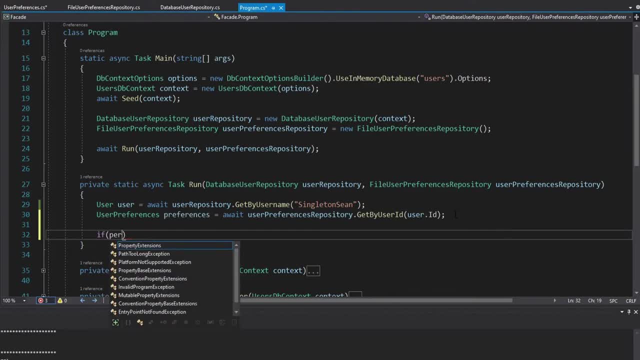 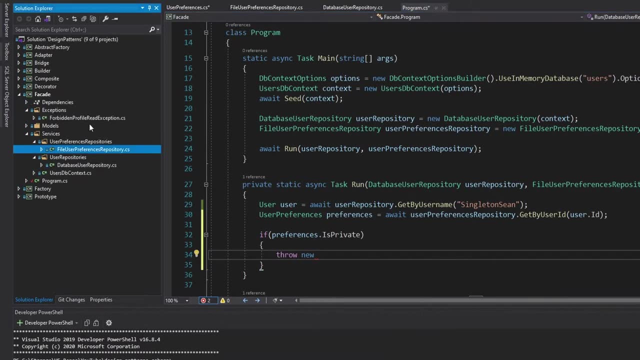 if the user's profile should be private- and that's in my preferences- and if the profile should be private, then we're going to throw an exception and the exception I have over here in my exceptions folder It's a forbidden profile read exception, so we're not allowed to view this profile. but if we can read, 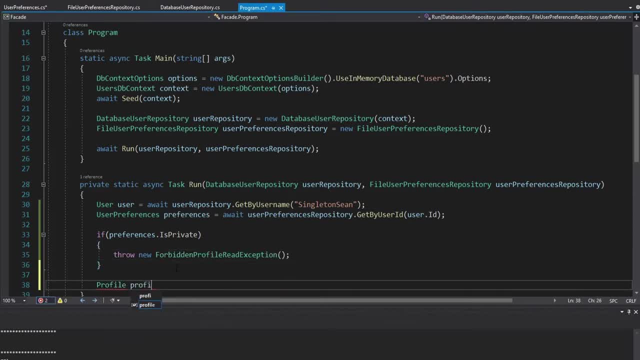 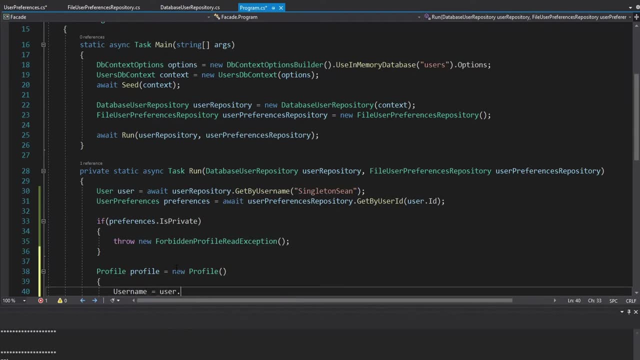 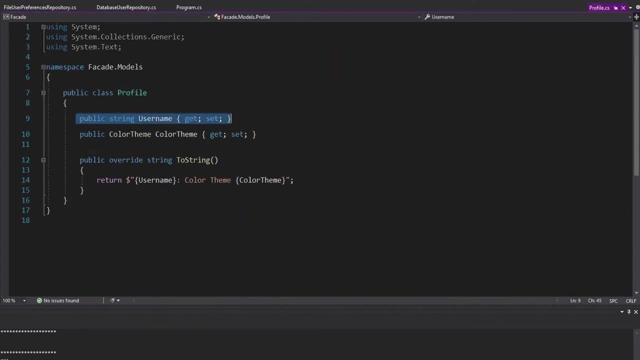 the profile, then we are going to create that profile. so I have a profile model. I'll show that off in just a second. but that takes in the username which we have on our user and the color theme which we have on our preferences. and if we look at our profile model, all we have is the username and 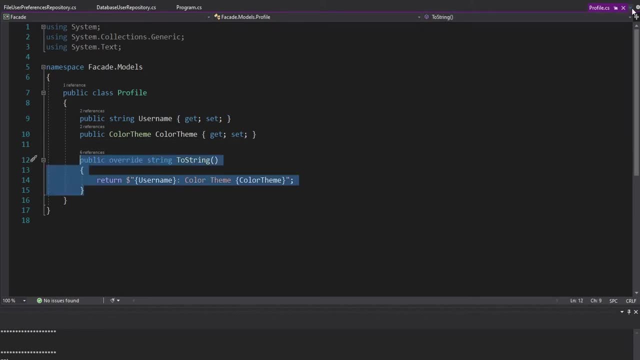 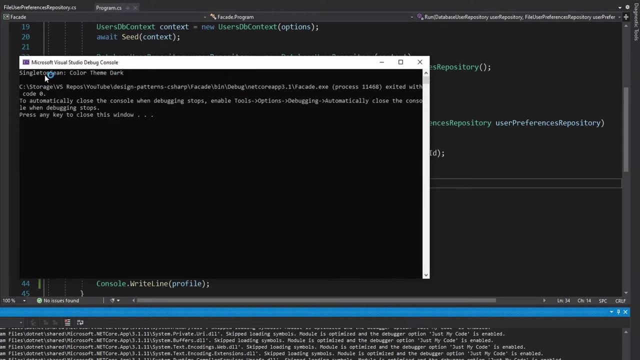 color theme and also a toString override, which we'll see in just a second, because now all we're going to do is write the profile to the user, the console, and let's see this in action. and there we go. there is my profile, so there's my. 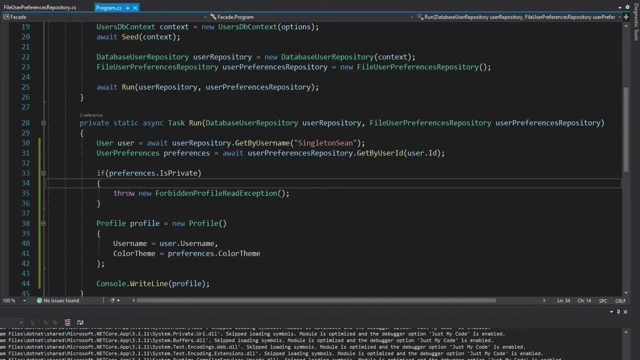 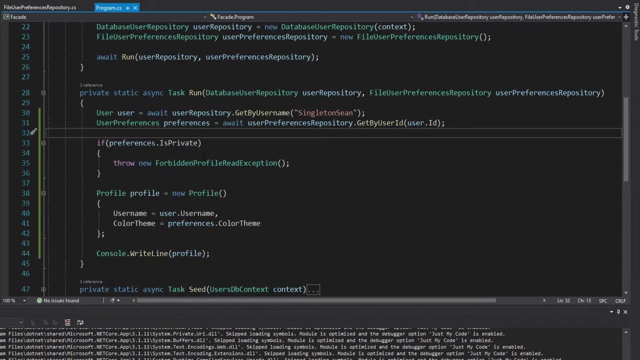 username and my color theme. but the issue we have here is that our programcs, and specifically this run method, that is essentially our client, and our client is doing way too much just to write a profile to the console, so it has to get the user. then the user's preferences check if their. 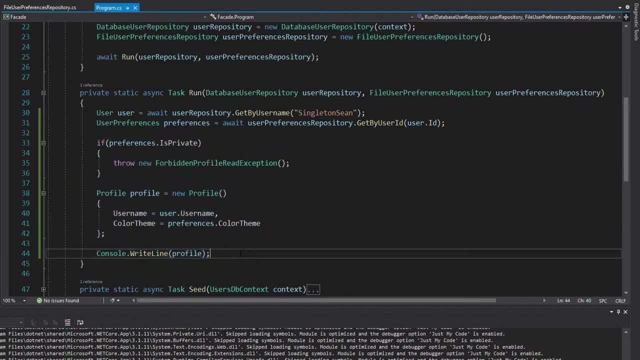 profile is private, create the profile, blah blah blah and then right to the console. ideally, all the client needs to do- which is this run method- is just get the profile by the user's user profile username. so we're going to create a facade to satisfy that functionality and then the client 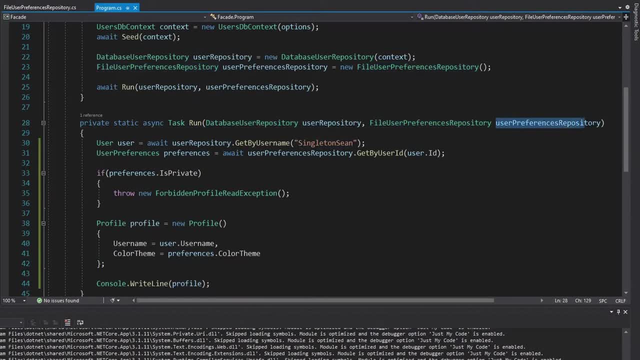 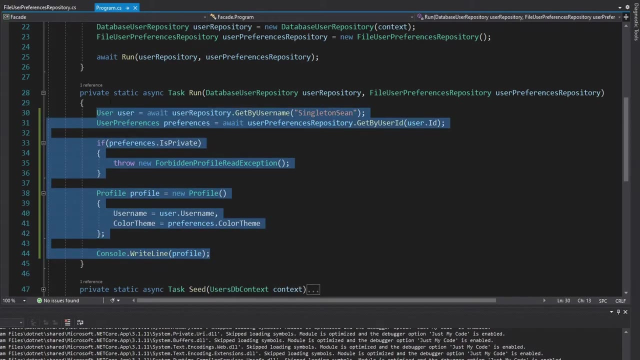 isn't going to have to know about the user repository, the user preferences repository. all it can do is use the facade and get the profile by the user's username. and again, the benefits of that are adhering to the single responsibility principle. so our facade will be responsible for bringing our subsystems together, and then our client will be responsible. 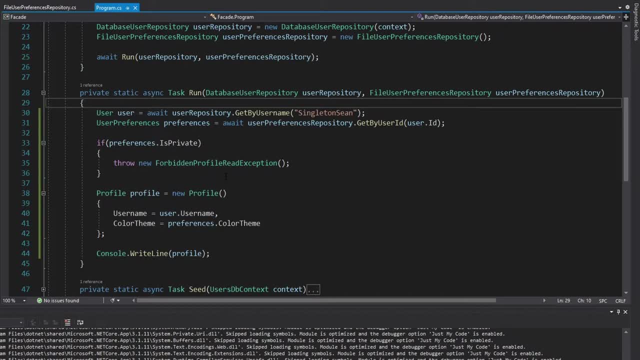 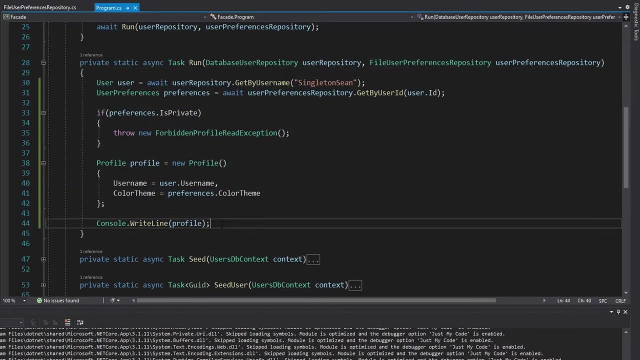 for just running the application and getting the profile for whatever user we want. and another benefit is, since all of this subsystem interaction will be moved into a facade rather than just baked into this run method, it's going to be much more reusable because we can just reuse the facade wherever we need to get a profile. so, for example, if we had like 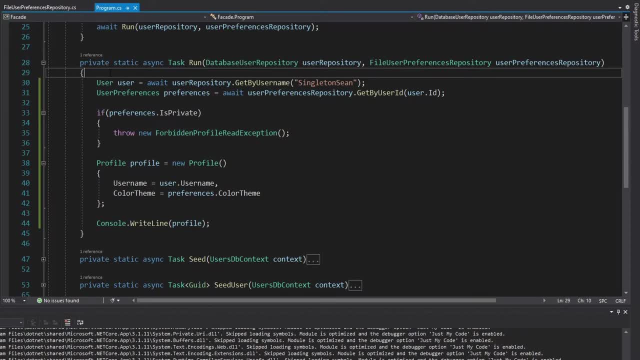 an aspnet core web application and we needed this logic inside of a controller method handler instead of just copy and pasting this, which would be terrible. we're going to have this in a facade, so we can just reuse the facade between the two of them. 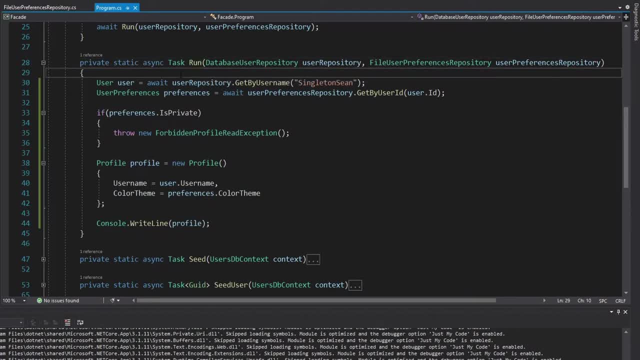 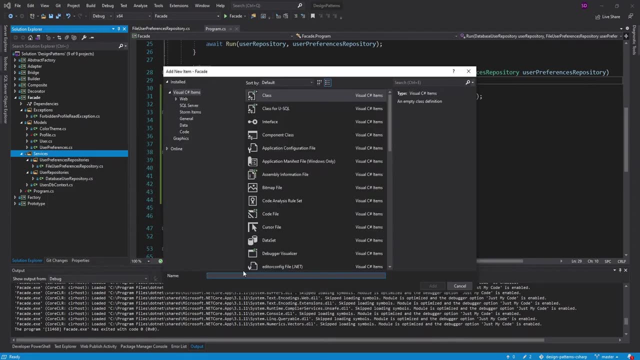 anyways, let's make that facade. so i'm going to create a new class over here. and for naming this, let's think about what our facade is going to do. well, it's going to read a profile, so i'm going to call it the profile reader. i guess you could call it something like the profile reader facade, and 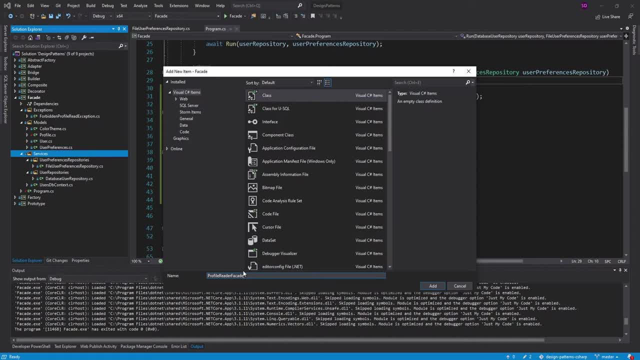 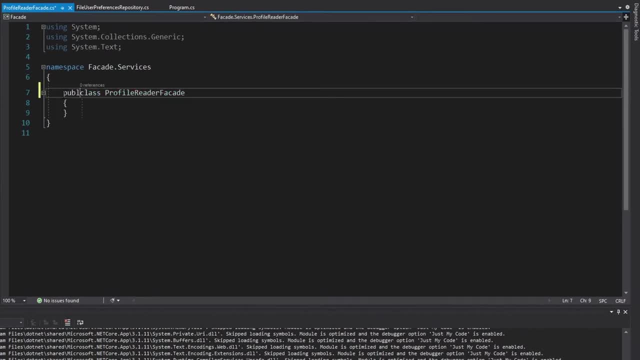 maybe i'll do that for this demo. just to point out that this is the facade. i'm going to do that, but probably in my own application i'll just call it the profile reader. we don't necessarily have to enter the name. so our facade is bringing subsystems together, so we're going to need 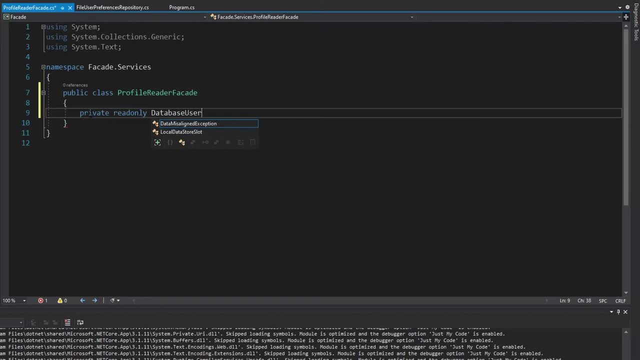 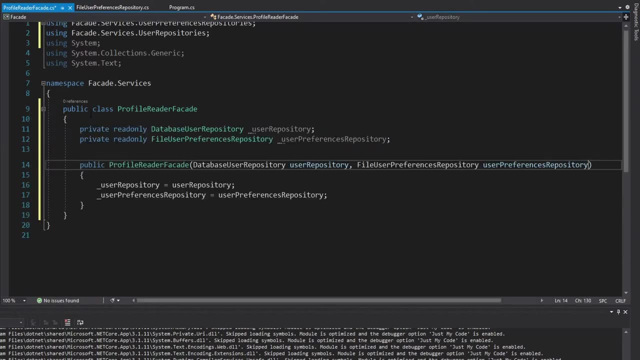 those subsystems as fields in this class. so first the database user repository and then the file user preferences repository, and then generator constructor for those. and now what is our profile reader facade going to do? it's going to read a profile by a user's username. so i'm going to have 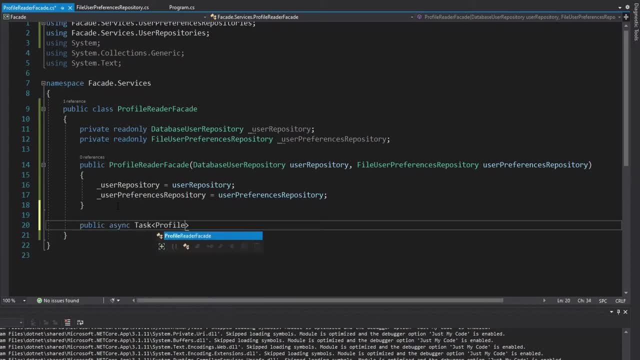 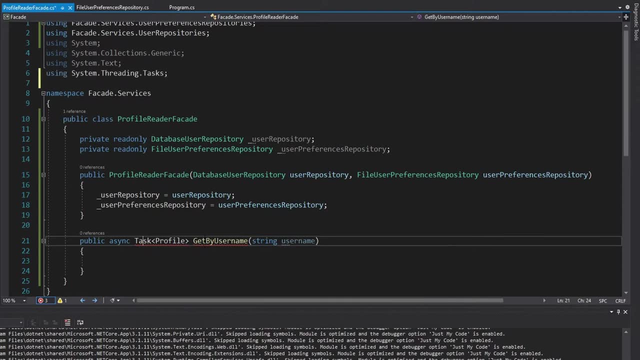 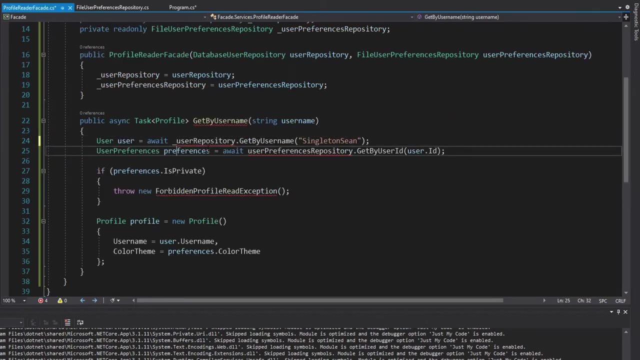 a single method on here that will return a profile- and i'll simply call this git by username- and that will return a profile. we want to get: import everything we need. and now for this method, we can just grab this from our programcs. so just cut this all out, rename our variables, import the. 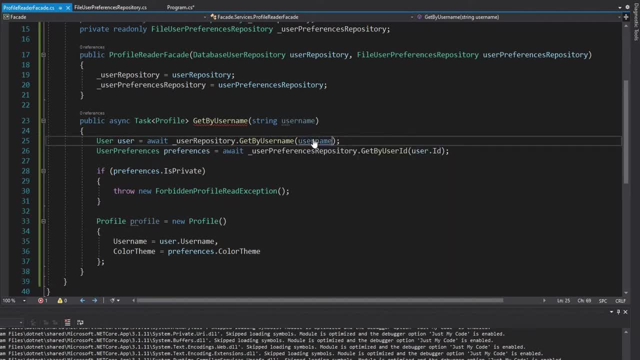 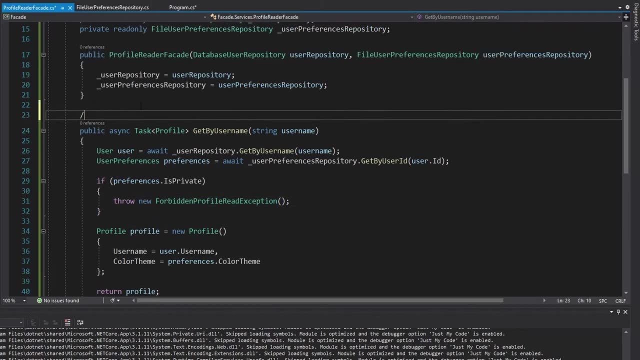 exception. make sure we pass in our username rather than the hard-coded singleton sean. there we go and then return the profile at the end of the method. and since we're throwing an exception in here, i love to document my exceptions, so we will do that, i guess. first, document the. 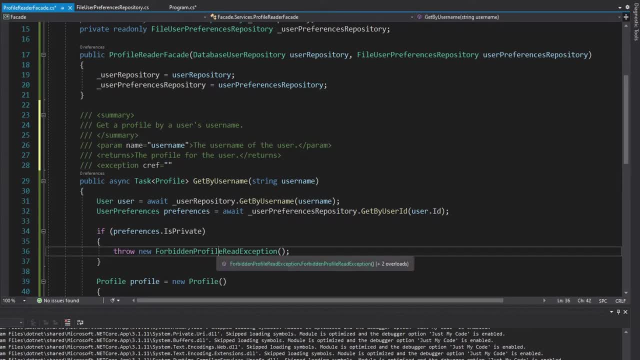 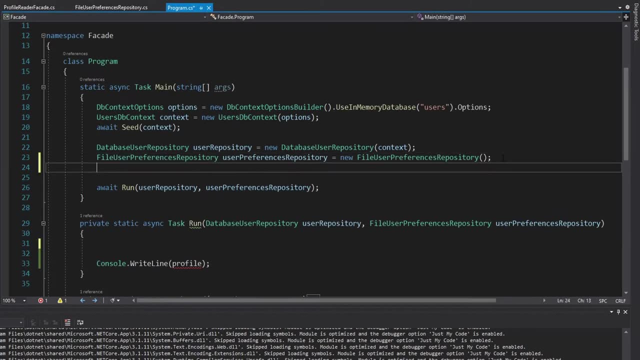 entire method and then document the exception. this is a forbidden profile that is thrown if the profile is private. and now back in the program with cs. let's set up our facade, so instantiate that up here and that'll take in the user repository and the user preferences. 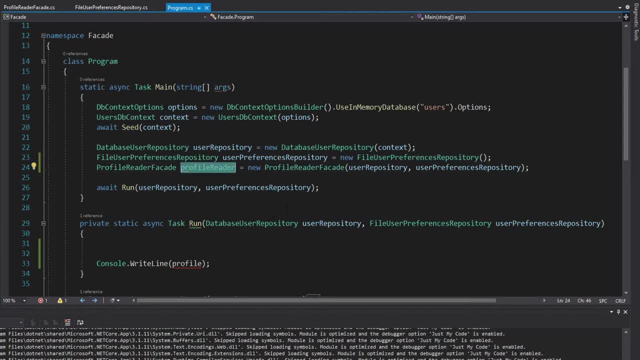 repository, and now what we're going to do is pass the profile reader to our run method. so this is going to change and update our method parameters down here. so another great thing about the facade pattern is now our run method just takes in this single parameter. so since we unified our subsystems, 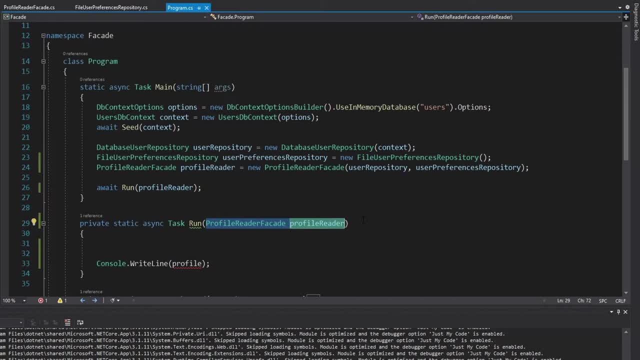 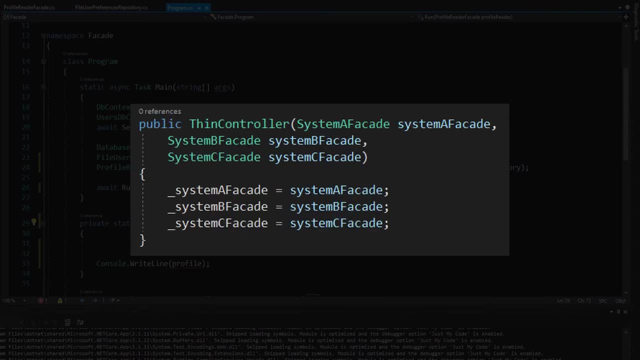 there's only one class that we have to deal with, so this pattern is also great. if you notice your constructor is getting gigantic or you have a method that takes in a bunch of different services, then maybe that class or method is doing too much and you could use a facade. and that's what we're. 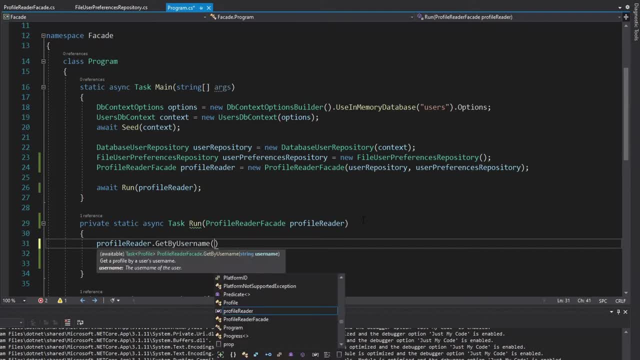 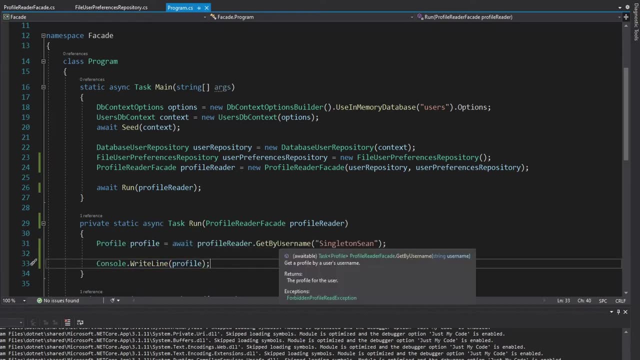 going to do? we're going to use this facade and get a profile by a username and we want singleton sean's profile, await that- and then we'll simply write that profile to the console. but if i look at this method, we see there is a forbidden profile- read exception. so we're going to catch that good. 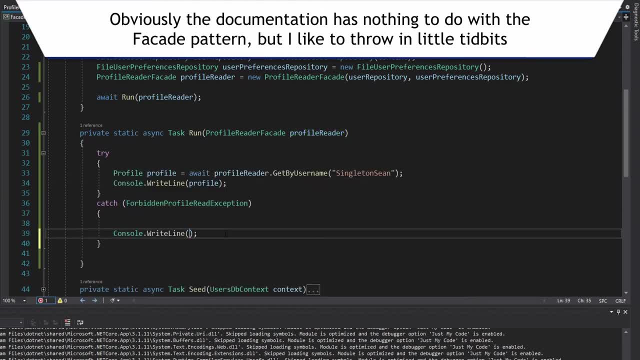 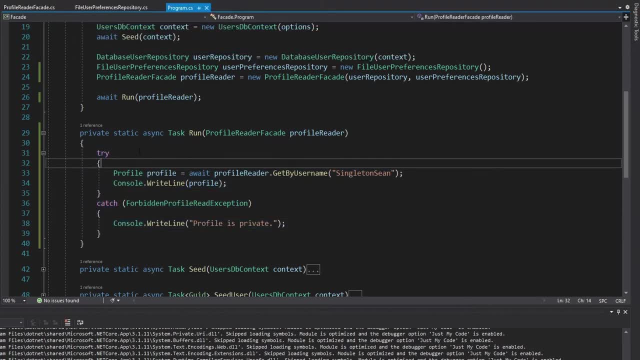 thing. i had that documentation that i could remember that exception. and if we catch that exception, we're going to say: profile is private. and now, as we can see, this run method is much simpler, but it's still just as powerful as before. does the same exact thing. let's see that in action. and there is our profile. and now let me 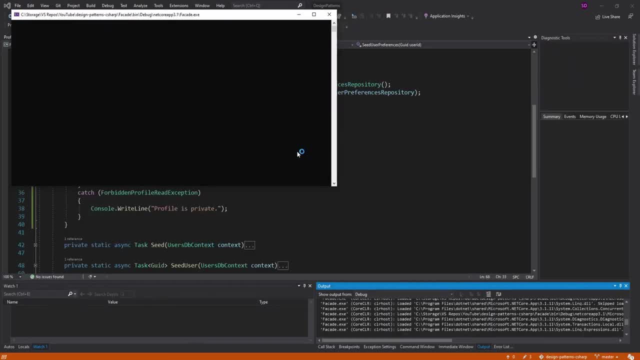 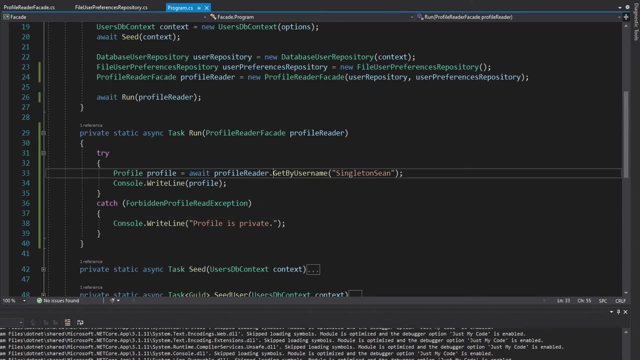 change my profile to private. try this again and we should get. the profile is private. so now we have this much simpler profile reader facade interface and all we have to do is get the profile by username rather than having to deal with the profile reader interface. and we're going to. 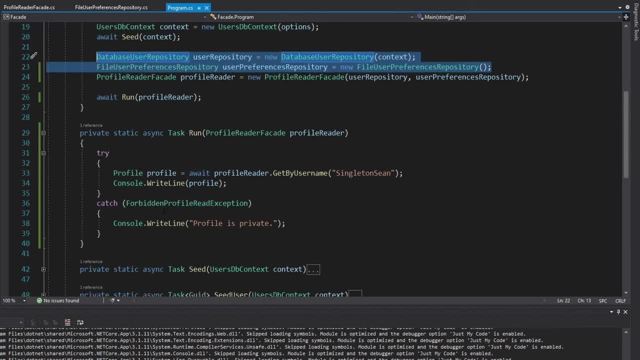 do that as well. we have a class here method that reallydrive this method, as well as a class here method where you can now actually go with all of our subsystems right here in the run method, so we can reuse this facade wherever we want for any client, and they're going to be pretty happy because